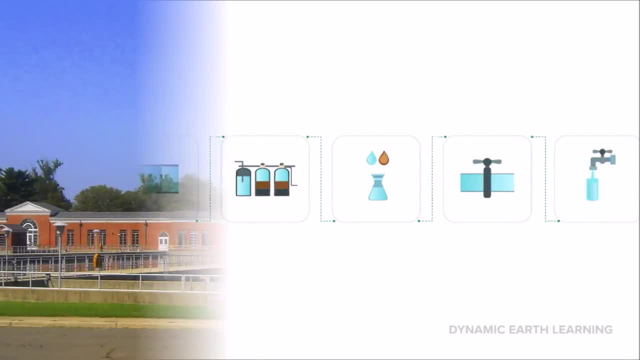 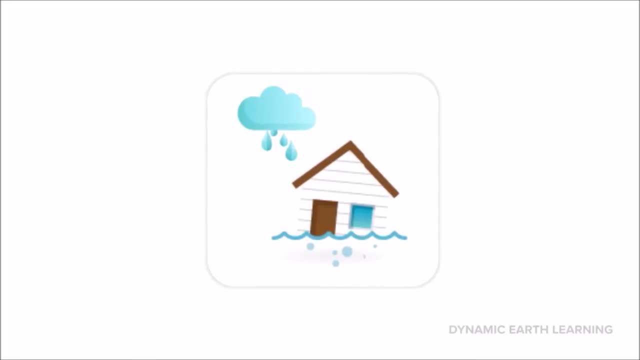 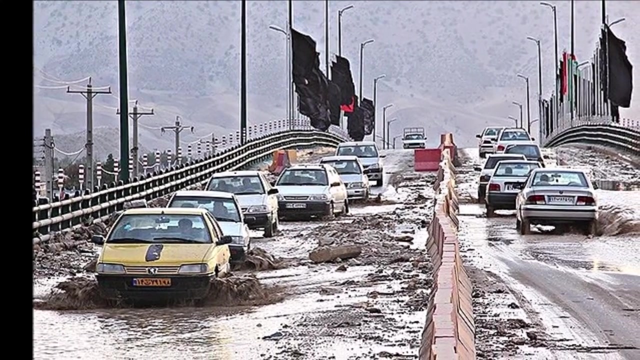 Reservoir water can be used to supply water to our homes and factories after it is sent to special treatment plants to make it safe for drinking. Flood control Reservoirs can prevent downstream flooding by maintaining and regulating the water flow during floods. They also balance water. 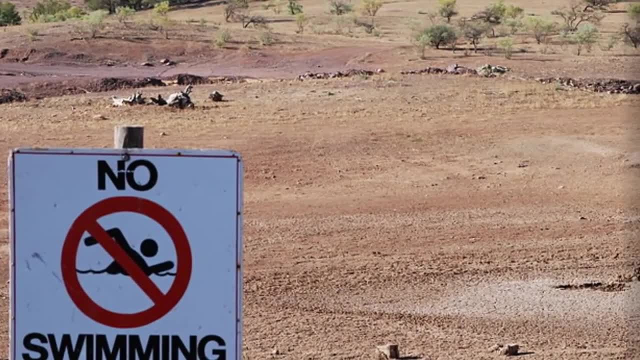 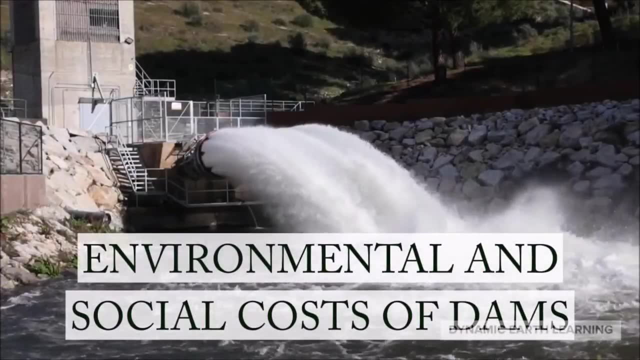 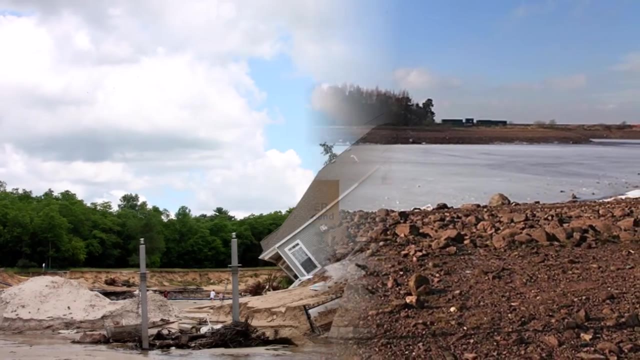 flow based on weather conditions, by holding water back during heavy rains and releasing more during a dry spell. Environmental and social cost of dams. Dams and Reservoirs are created to provide a benefit to people, but they can also have a disastrous impact on our environment People. 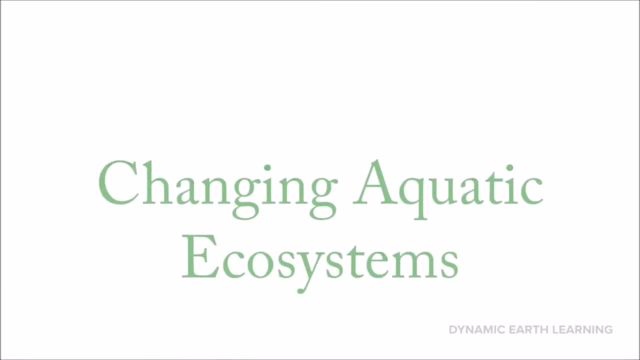 that live close to dams are especially impacted. Environmental impacts include changing aquatic ecosystems. Building a dam in a river leads to vast changes in aquatic life, Water quality, water bonded nature and life. Water quality flies through freshwater pipes, evokes a water representatives For better or for worse. sometimes, conservation of artificial water comes first. 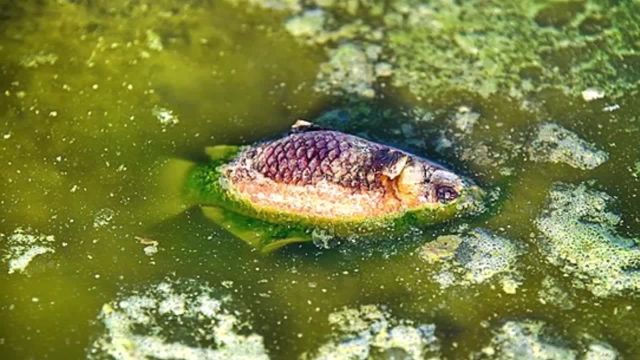 Also reservoirs can work. Bey on theródrage, счит mes corimeteria y calidad al tamar. or poisoned bas. beneath them, moored water, enfants in volcanic reservoirs, Water phenioxid canonizingatore Diego IPC이라고 Technologies Republic of China. These changes can. 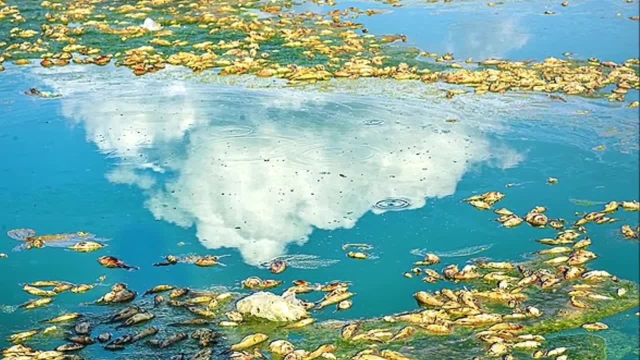 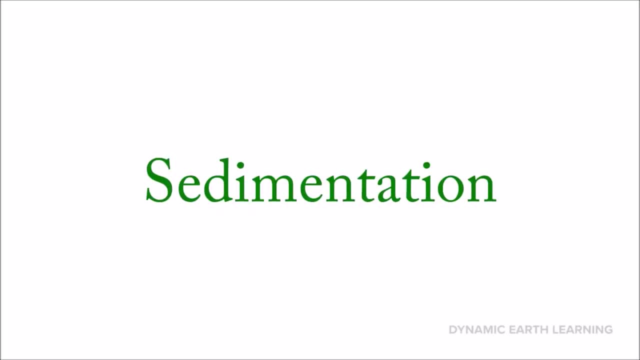 make it less suitable for certain fish, which eventually leads to the loss of some of the species or enables predators too easily reach them. What are Reservoirs? Dams and reservoirs can decrease biodiversity of an area As the flow of water decreases. 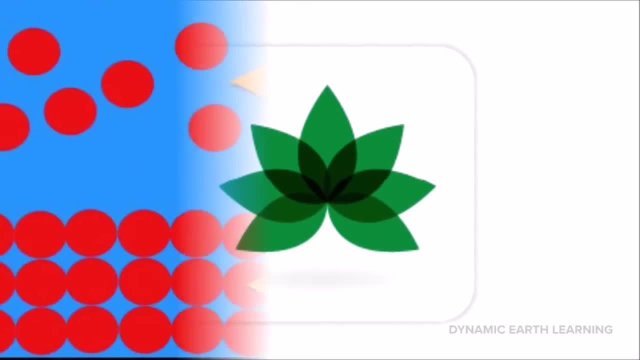 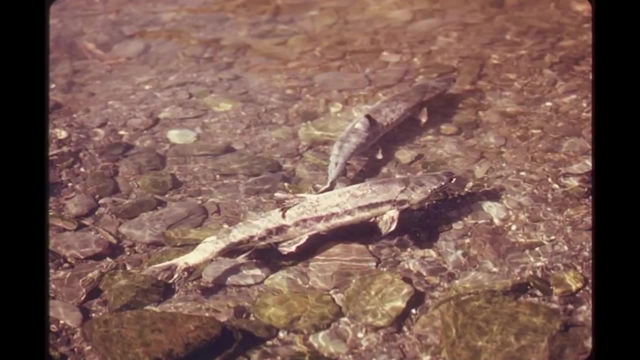 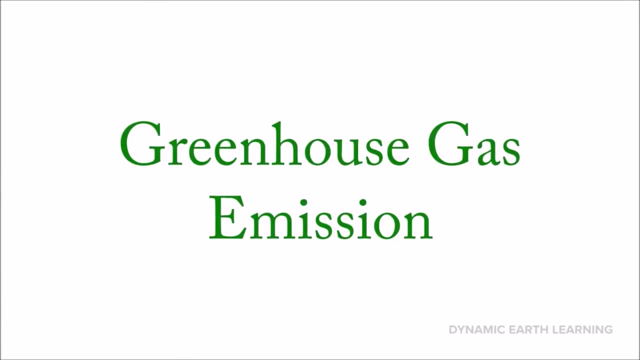 sedimentation increases. Now to set a B ingredients is when particles that would normally flow through an area get caught in one place and settle in the water. Sediment can bury rock beds where fish lay eggs or cover up other important food and habitat features. Greenhouse gas emission: The reservoirs cause rotting vegetation in the water Through the. 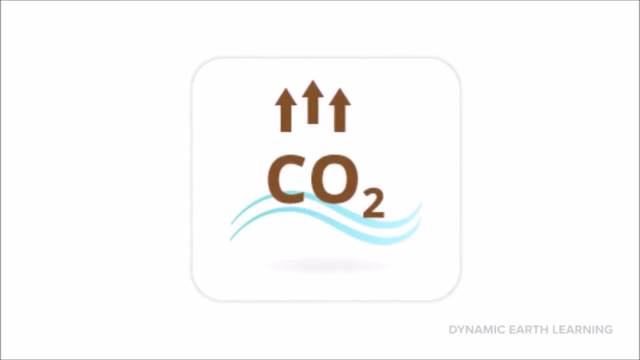 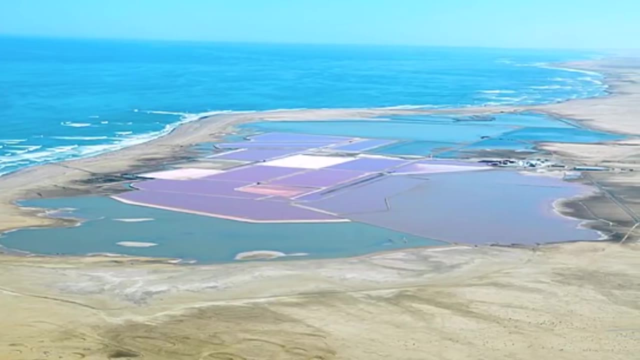 process of decomposition, the greenhouse gases methane and carbon dioxide are released. Evaporation- Open surfaces of the reservoirs speed up water loss by the evaporation process. Generally, much more water is lost from reservoirs than is lost from the flowing rivers they replace. 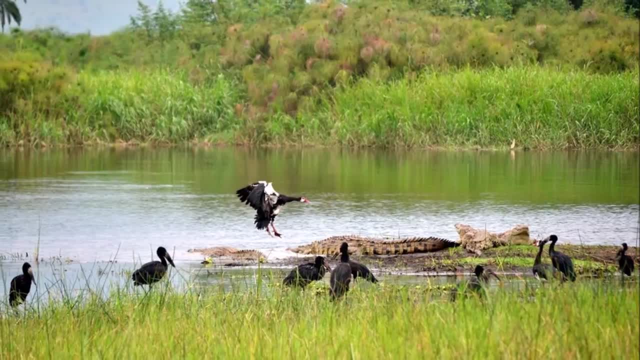 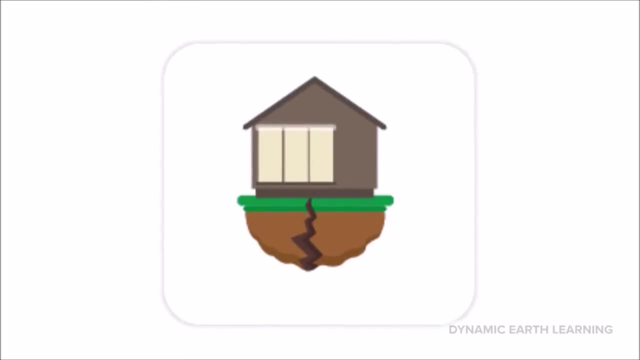 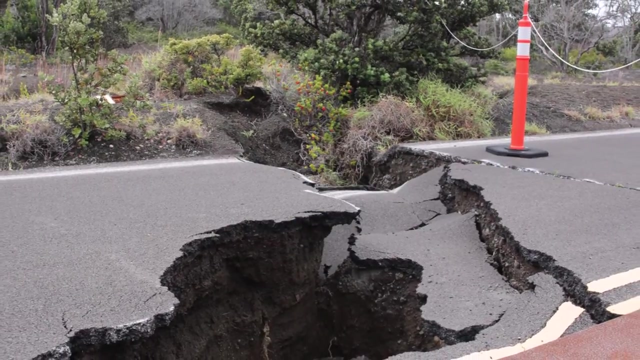 Increased evaporation can affect the microclimate and ecosystems of an area. Seismic activity: Did you know that larger dams can trigger seismic activity or earthquakes? This is due to changes in the stress of the weight of water or increased ground pressure that decreases the strength of rock under the reservoir.